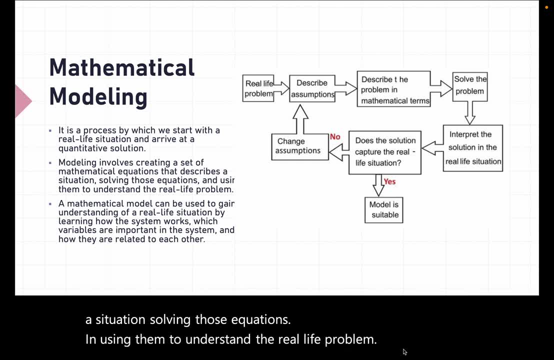 real-life problem. A mathematical model can be used to gain understanding of a real-life situation. by learning how the system works, which variables are important in the system and how they are related to each other, Mathematical modeling can help predict the future. So in the figure to the right it describes a model of a real-life problem. 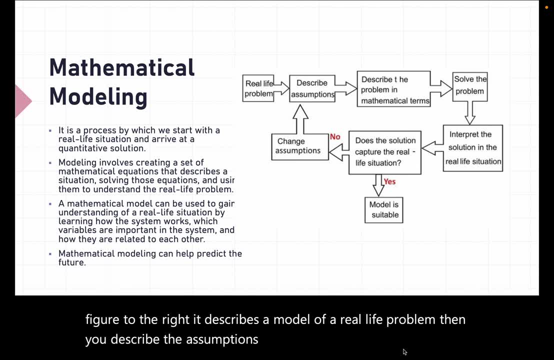 then you describe the assumptions, you describe the problem in mathematical terms, then you solve the problem, You interpret the solution in a real-life situation and then you ask yourself: does this situation, does the solution capture the real-life situation? If yes, then your model is suitable. If no, then you need to change your assumptions and you need 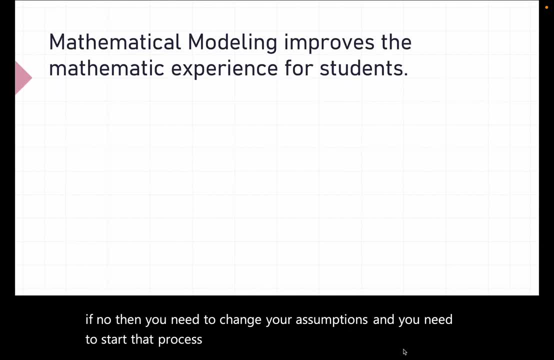 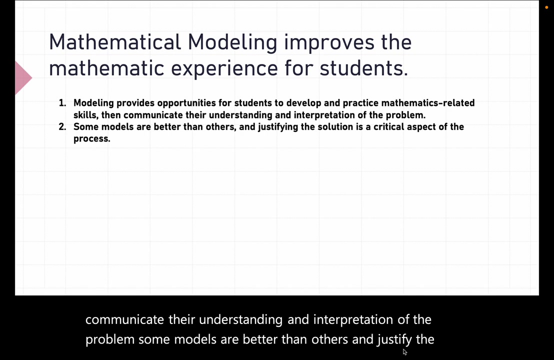 to start that process, to refine that mathematical model. Mathematical modeling improves the experience for futures. Modeling provides opportunities for students to develop and practice mathematics-related skills, then communicate their understanding and interpretation of the problem. Some models are better than others and justify the solution is a crucial 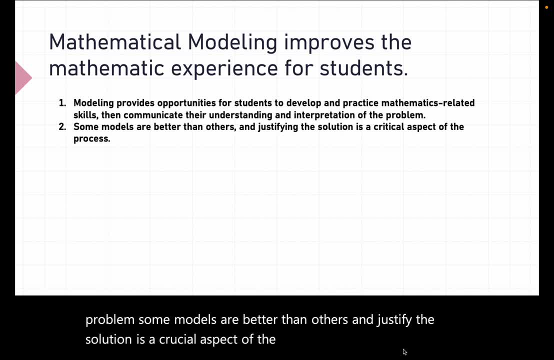 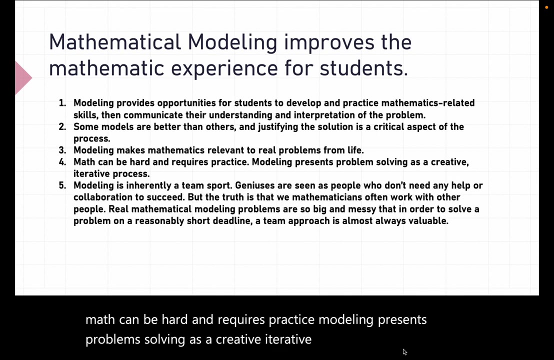 aspect of the process, so you must justify your solution. Very crucial, Modeling makes mathematics relevant to real-world problems for life. Math can be hard and requires practice. Modeling presents problems solving as a creative, iterative process. Modeling is inherently a team sport. Geniuses are seen as people who don't need any help or 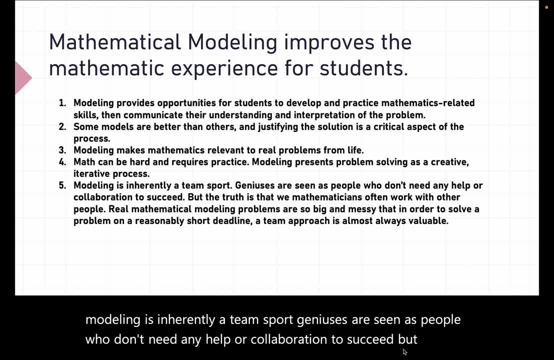 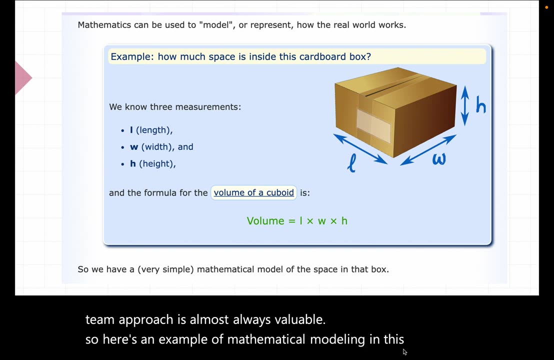 collaboration to succeed. But the truth is we, as mathematicians, often work with other people. Real-life mathematical modeling problems are so big and messy that, in order to solve a problem on a reasonably short deadline, a team approach is almost always valuable. So here's an example of mathematical modeling. In this picture, mathematics can be used to model. 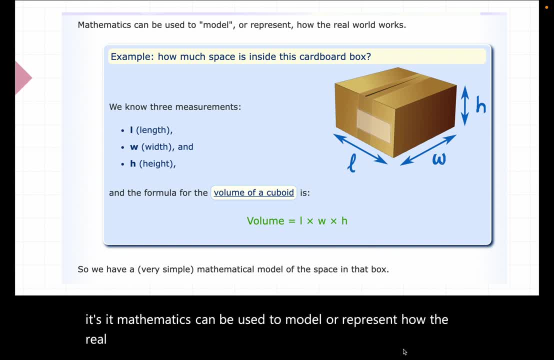 or represent how the real world works. So in this example, it wants to know how much space is inside this cardboard box. So we know that the real world works. and we know that the real world works, So we need to use the length, the width and the height, those three measurements, And we 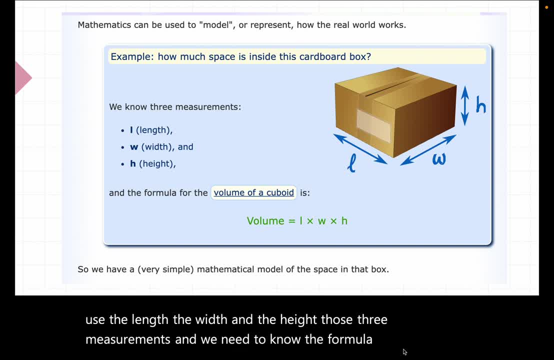 need to know the formula volume of a cube, or a square in this case. So you would multiply the length times width times the height. This is a very simple mathematical model of the space in that box. However, this problem can actually get a little bit more complex because then, once you 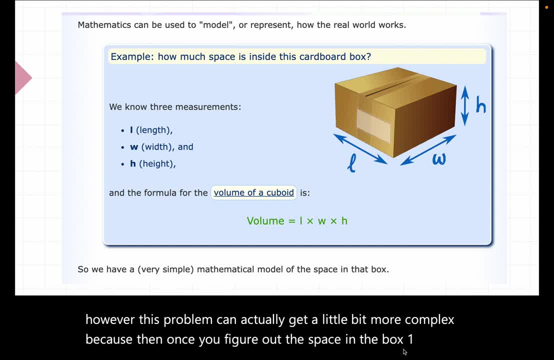 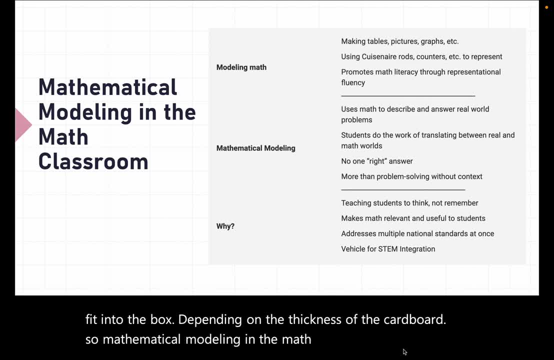 box? Well, you might think, well, how thick is the cardboard box? Well, you might think, well, how thick Mathematical modeling in the math classroom, many teachers do this on a daily basis. With math modeling, you're making tables, pictures, graphs. 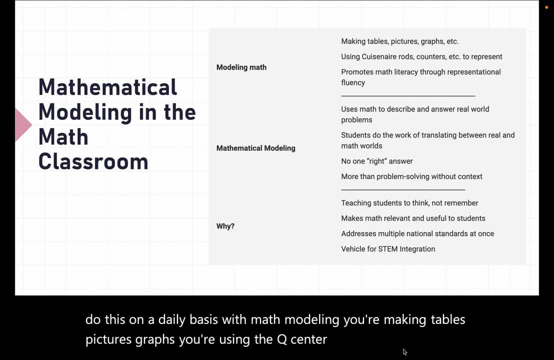 You're using the Cuisinart rods counters- anything to represent any type of modeling situation. You're promoting math literacy through representational fluency. Mathematical modeling uses math to describe and answer real-world problems. Students do the work of translating between real and math worlds. 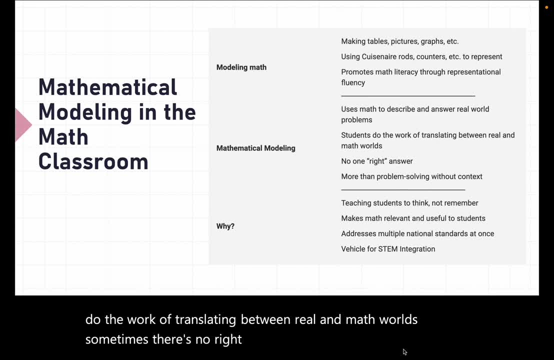 Sometimes there's no right answer more than problem-solving without context. Why Teaching students to think and not remember is a great reason why It also makes math relevant and useful to the students. It addresses multiple national standards at once and is a vehicle for STEAM integration. 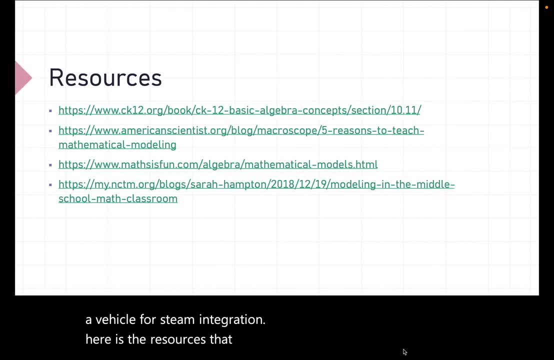 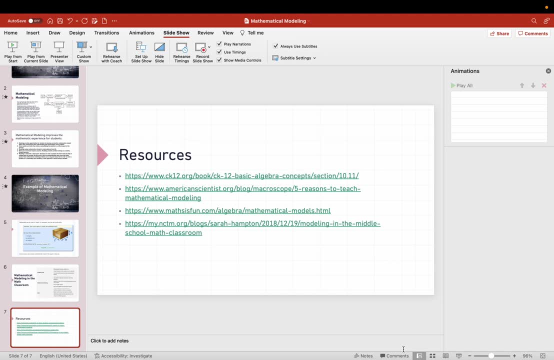 Here is the resource. Here are some of the resources that I used in order to create this video. Thank you for watching my show and have a wonderful day.